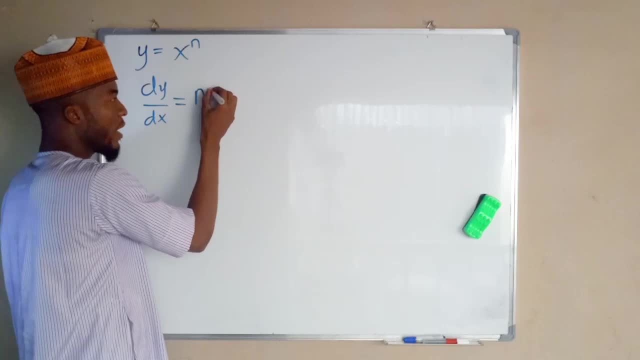 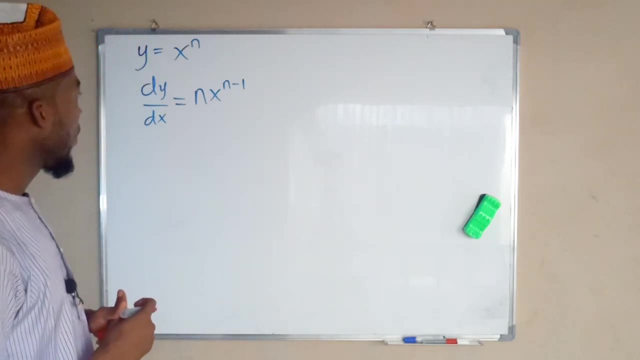 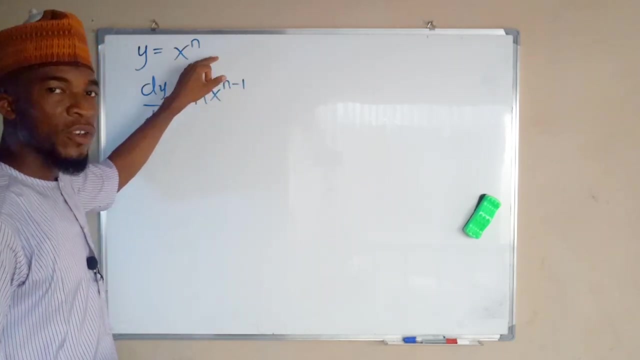 here, f of x is equal to nx, to the power of n minus 1, this is what we have learned in our previous lesson. integration is telling us that if we integrate this function, we are going to get back our original function. Everything you do in differentiation, you have to do the opposite. 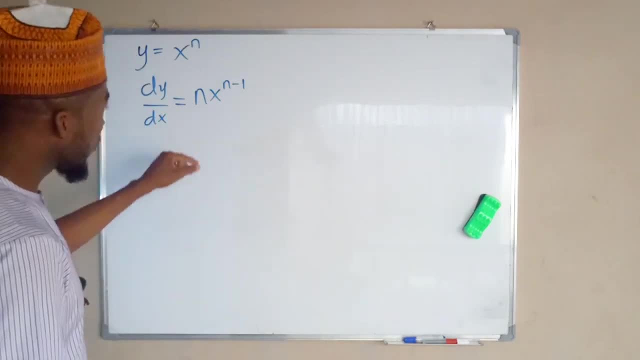 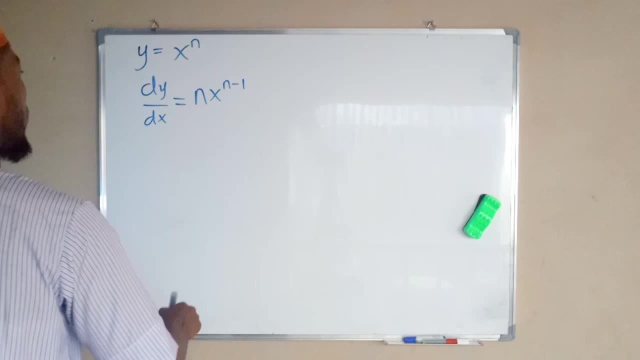 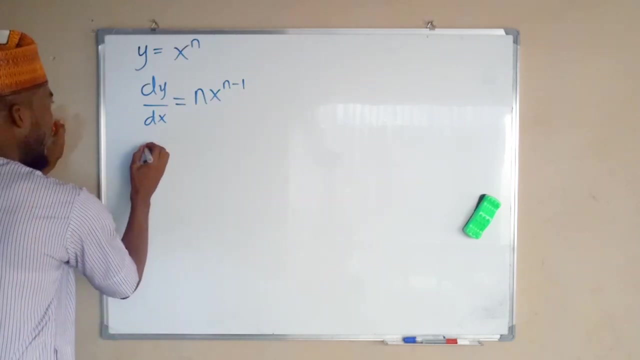 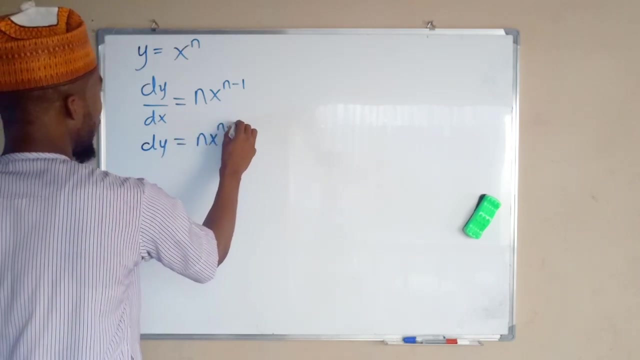 of that in integration. alright, let us now integrate this function to see whether we are going to obtain this function, our original function. What we are going to do now is to multiply both sides by dx, thereby obtaining dy equals nx to the power of n minus 1 dx. So now we are going to 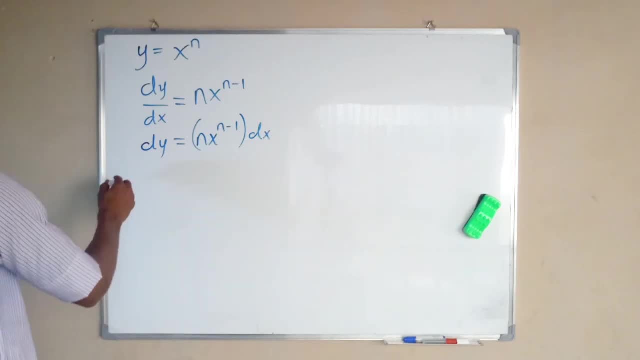 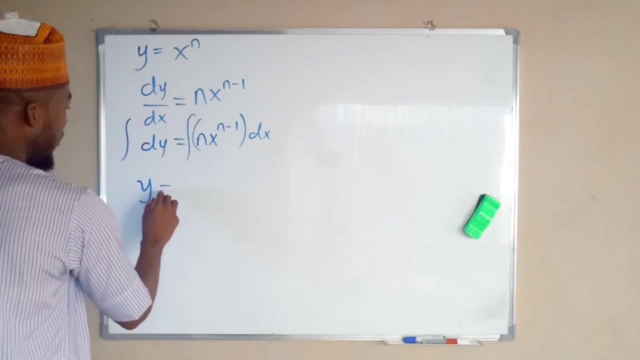 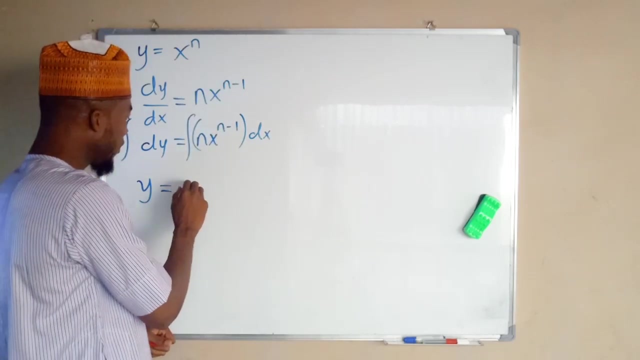 integrate both sides. by integrating the left hand side- and this is the sign of integration- We also have to integrate the other side with respect to x. By integrating the left hand side, we are going to obtain y, and to the right hand side, look of Whatever we do here, we are going to do the opposite. So this is: 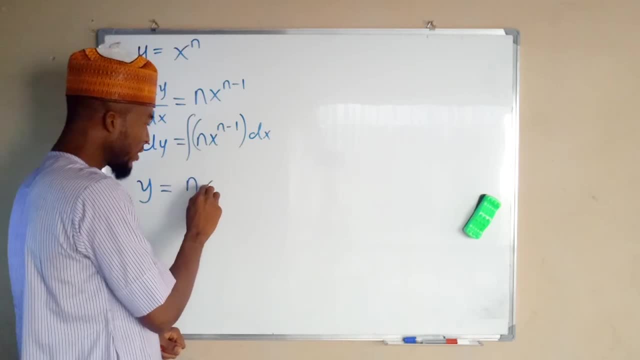 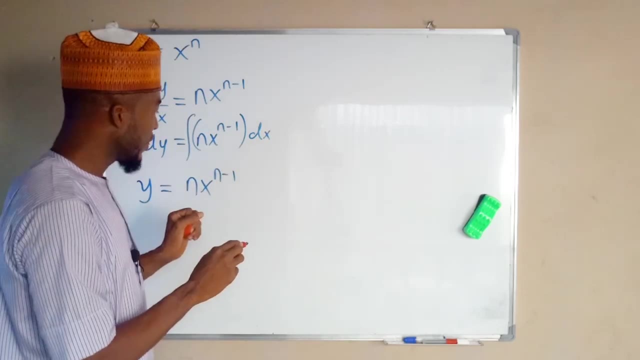 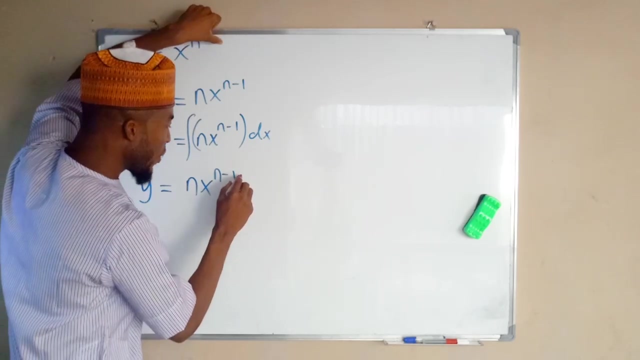 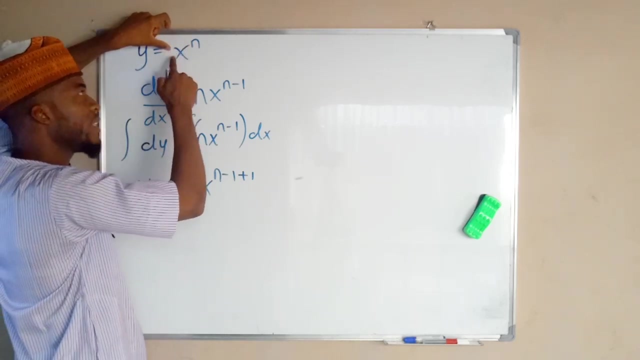 equal to nx, to the power of n minus 1.. This is the function Now we are going to integrate. Remember, in differentiation we subtract one, but here we are going to add one. You see the opposite. In differentiation we multiply the function by the index, but 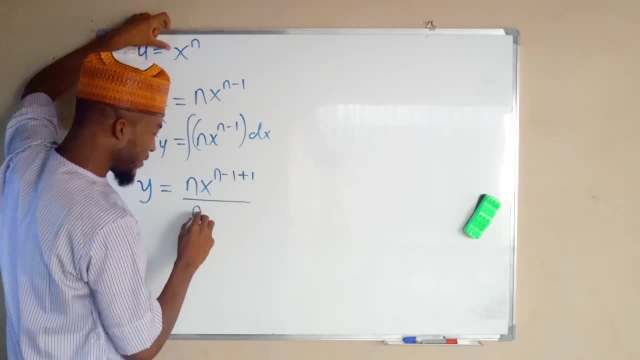 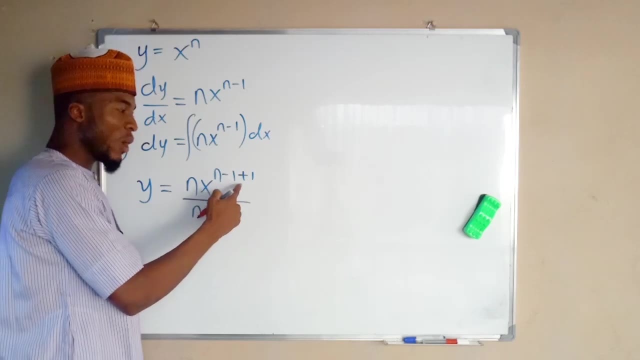 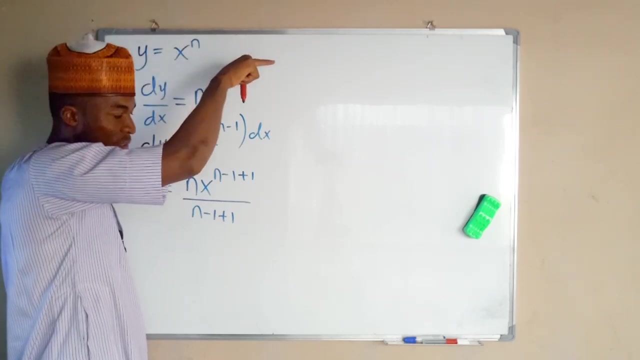 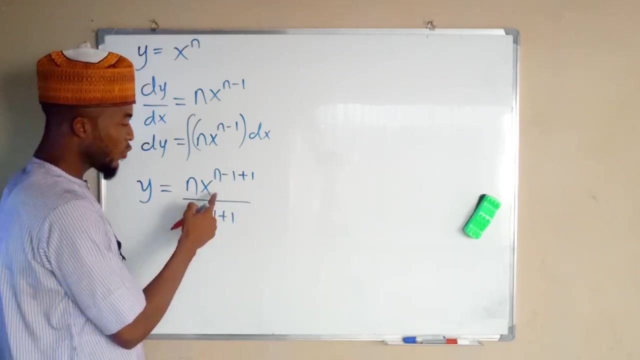 this time around we are going to divide by the index, and now the index is n minus 1 plus 1.. In integration you have to add before dividing, But in differentiation you have to multiply before subtraction. So now let us simplify: Minus 1 plus 1 is 0. So we have only n. So this is the same. 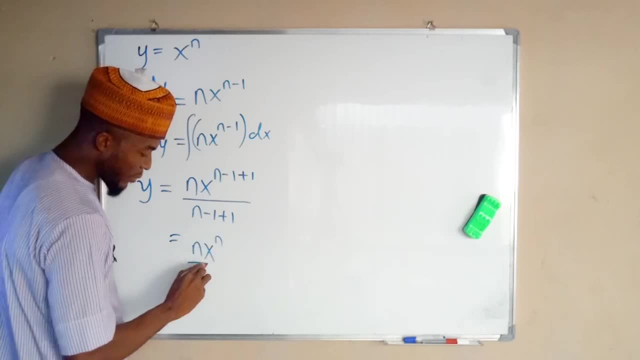 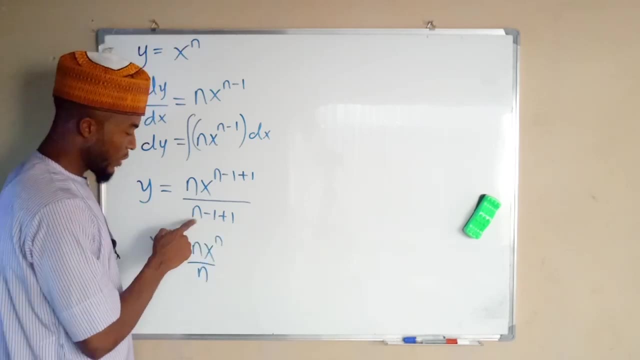 thing as n. x to the power of n. divided by This is the same thing as n. 2 plus minus 1 is 0, leaving only n And n. cancel n. Y- tir임 divide zero, leaving only n. So we have simple instruction: hw橡 minus 1 plus 1, 0, leaving only n and n. cancel n. Why do this? is required. 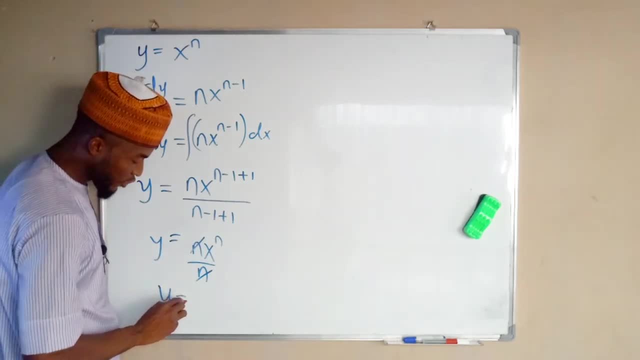 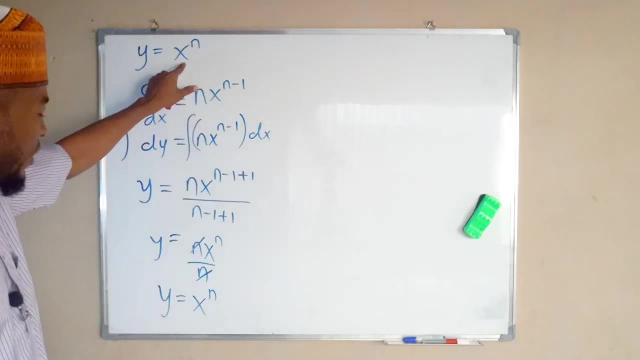 So this is the matrix For our destroyed function. we see thatünden it is true when the now equals to x, power, n. but in integration, you see, this is the function we have initially, but in integration we have to add a constant of integration, which is most often we use c and c. 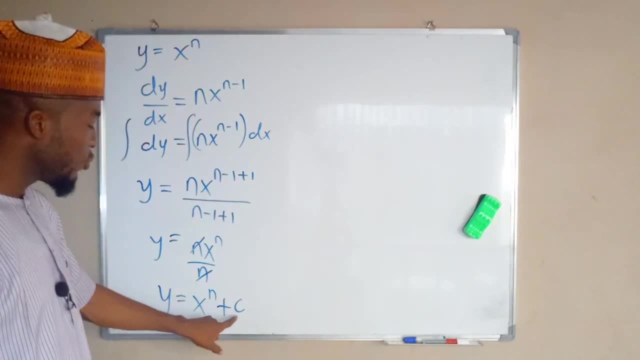 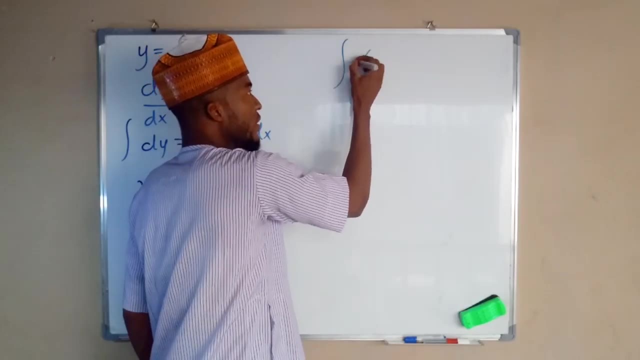 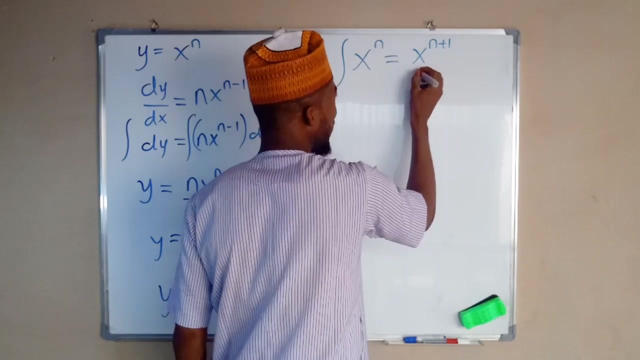 is a subset of real numbers. in my next example i will show you why we have this constant of integration. so, in general, if you want to integrate x to the power of n, this will be x to the power of n plus 1 divided by n plus 1 plus the constant of integration. so this is. 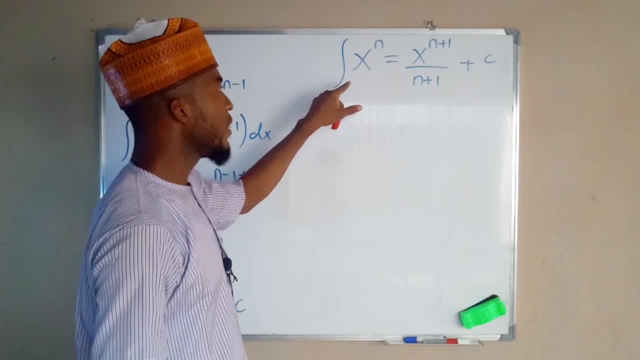 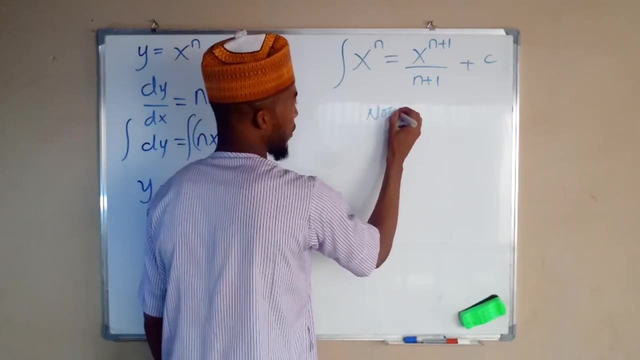 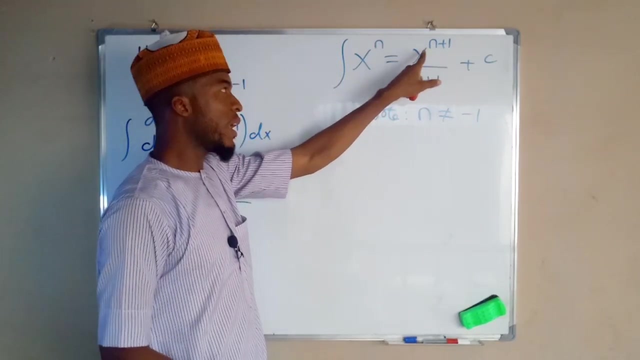 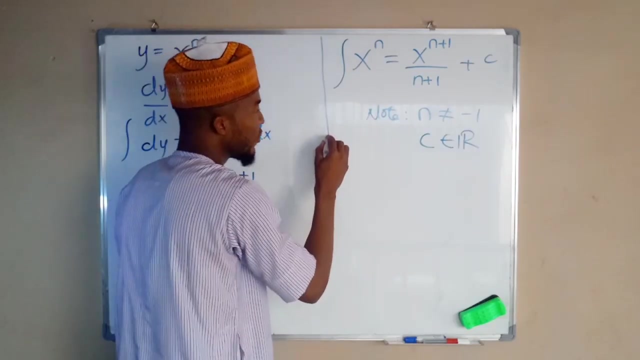 the formula we are going to use for integrating an algebraic function, but not n, is not equal to negative 1, because if it is negative, 1 plus 1 is 0 and x to the power of 0 is 1, then c, i told you, is a subset of real number. so this is the general form of integration. 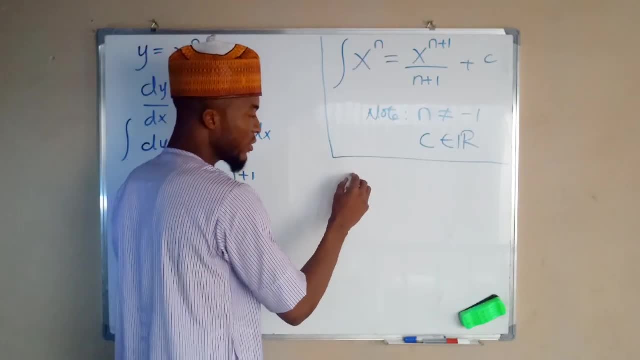 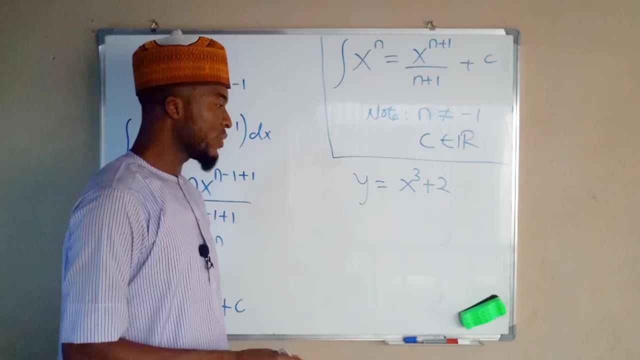 so now let us look on to another example. suppose y equals to x to the power of 3 plus 2. first of all, let us differentiate this function and see the result. by differentiating this function, we are going to see that x to the power of n is not equal to negative 1, because 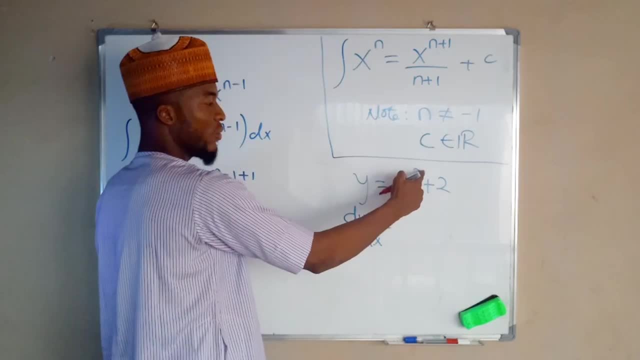 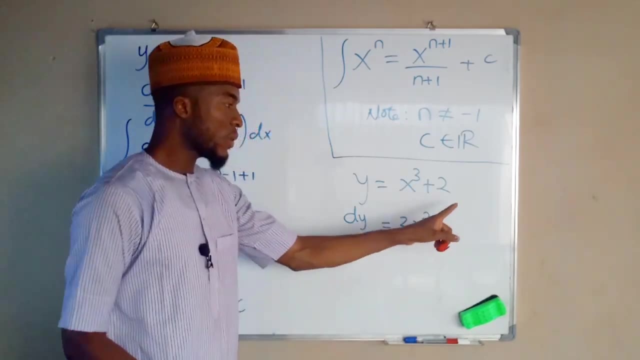 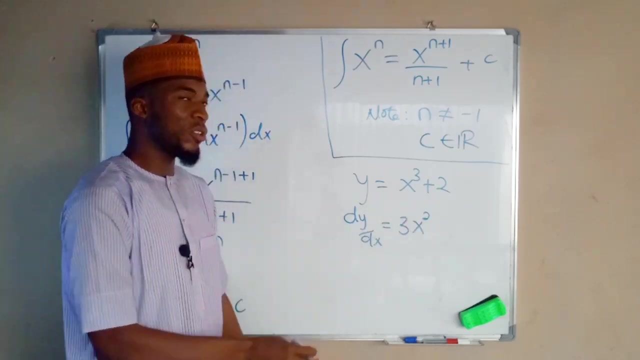 the function with respect to x, we are going to obtain- you know this exponent is going to come down 3, then you subtract 1 from that 2, the derivative of a constant term is 0. so this is what we have by differentiating this. so now let us integrate this function to see whether we are going to 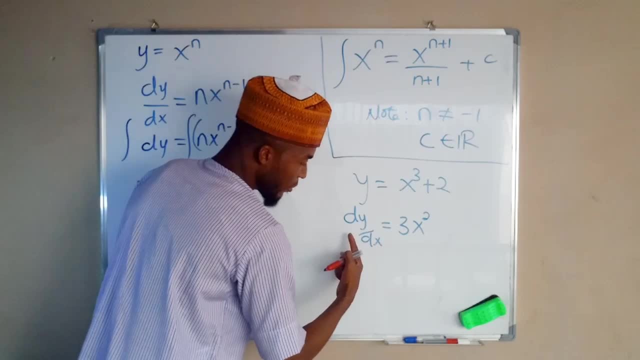 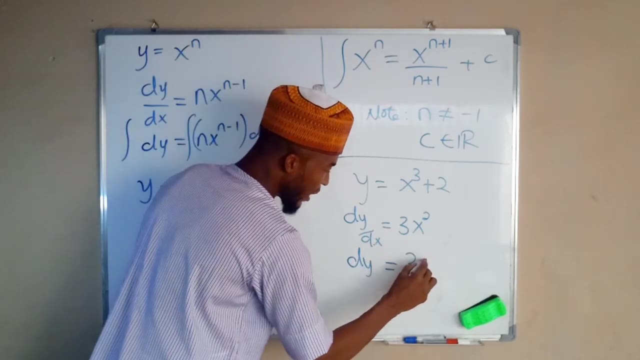 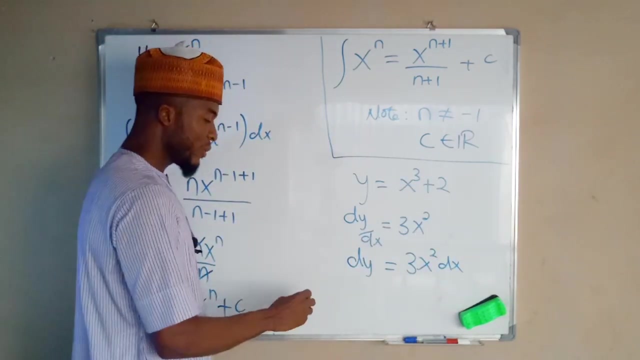 obtain the initial function. first of all, multiply both sides by dx so that we have dy on the left hand side and to the right hand side we have 3 x squared dx. let's apply integration to both sides, integrating the side, and to the other side too. 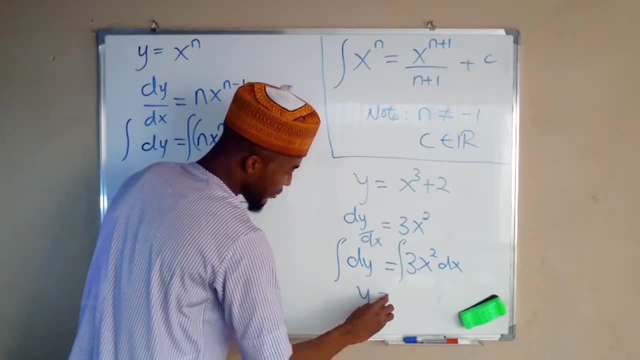 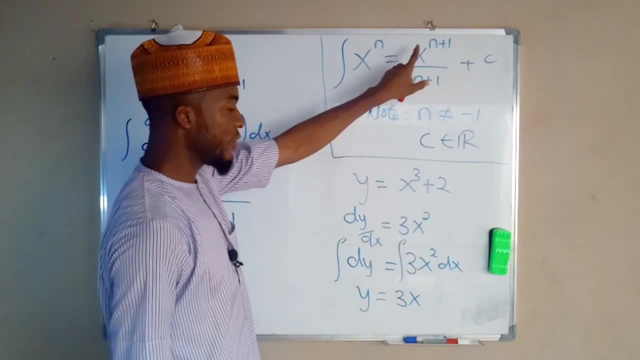 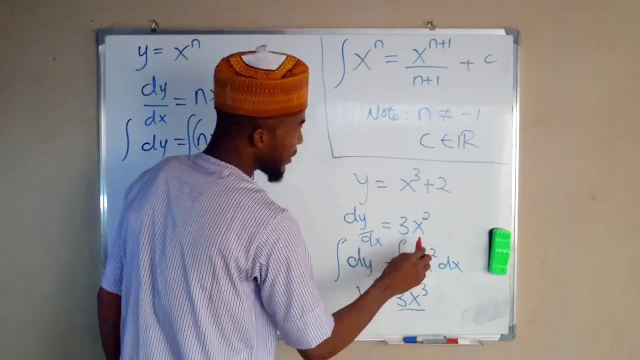 on the left hand side we have y, and to the right hand side we have 3 x. this time around, we are going to apply this principle. our index, which is n, is 2 plus 1, is 3. then divide by n plus 1, which is 2 plus 1.